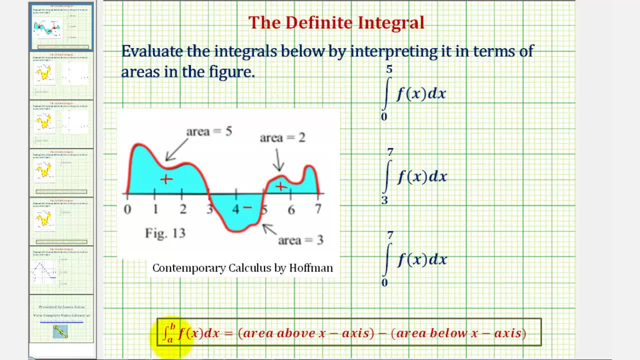 Another way to think of this would be: if we want to evaluate the def integral of f of x from a to b, we can take the area above the x-axis and subtract the area below the x-axis. So, looking at our first integral, we have the integral of f of x from zero to five. 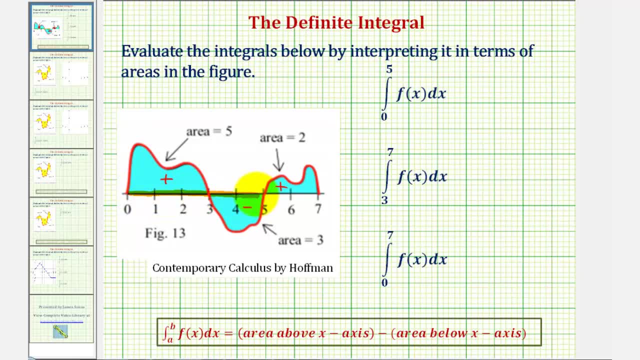 so we're integrating over this interval here where we have area both above and below the x-axis. So on the interval from zero to three the value of the integral would be positive five. but then on the interval from three to five, because the area is below the x-axis, 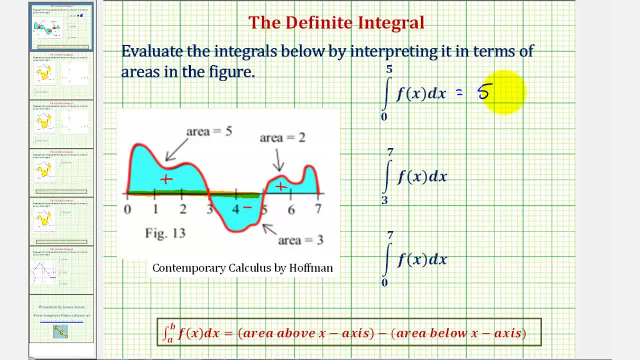 the value would be negative three. so we can either add negative three here or just subtract three, giving us a value of positive two. Next, we have the integral of f of x from three to seven, which would be from here to here. 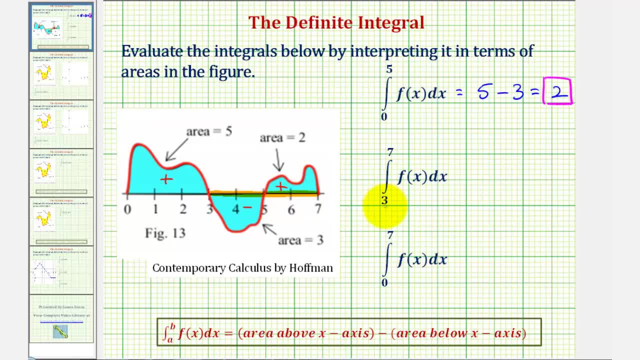 So notice, on the interval from three to five, the def integral would be negative three, because the area is below the x-axis. so we have negative three and then, plus, on the interval from three to five, the value of the def integral would be positive two. 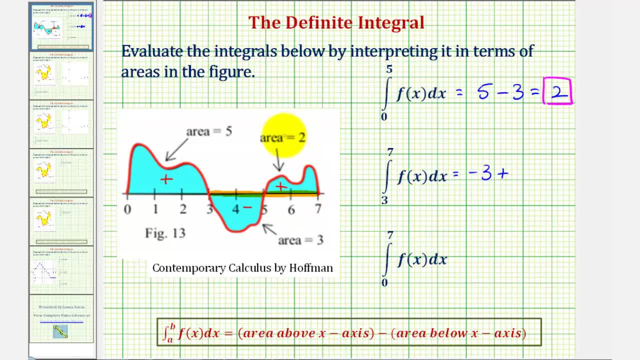 because the area is above the x-axis. So we have negative three plus two, which is equal to negative three, which is negative three, Which is equal to negative one. And then, finally, for the last integral, we have the def integral of f, of x, from zero to seven. 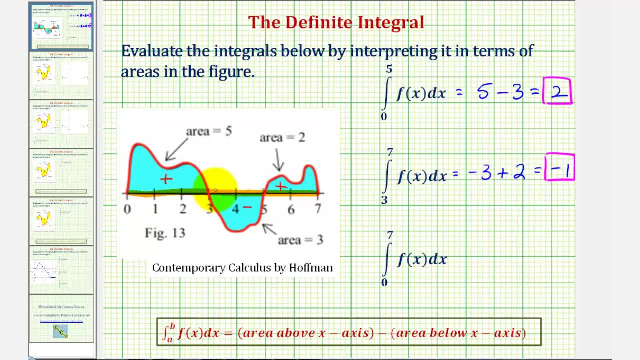 which would be over this entire interval here. So from zero to three, the value would be positive five because the area is above the x-axis. and then from three to five, the value would be negative three because the area is below the x-axis. 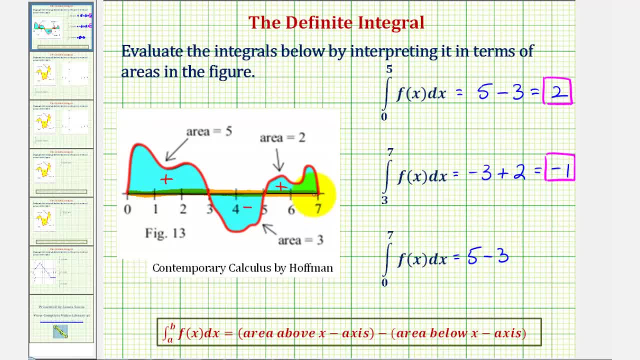 So again, we can add negative three or just subtract three, And then finally, from five to seven, because the area is above the x-axis, the value would be positive two. So we have five minus three plus two, which is equal to positive four.